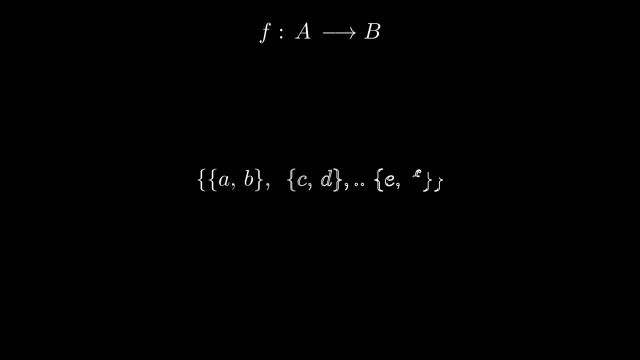 can be viewed as a set of tuples or other sets, where the first elements are taken from the domain and the second are functional values. Numbers are also sets. The naturals begin with the empty set. one is the set containing the empty set, and each next set contains all the previous ones. 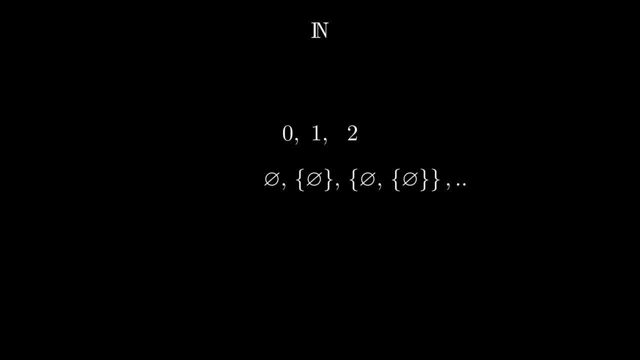 Likewise, the irrationals and irrationals have their set-theoretic interpretation. The particular set of axioms that we accept nowadays bears the name of Zermelo-Fraenkel. Most of them sound, reasonable and intuitive. Take extensionality: If two sets, A and B, 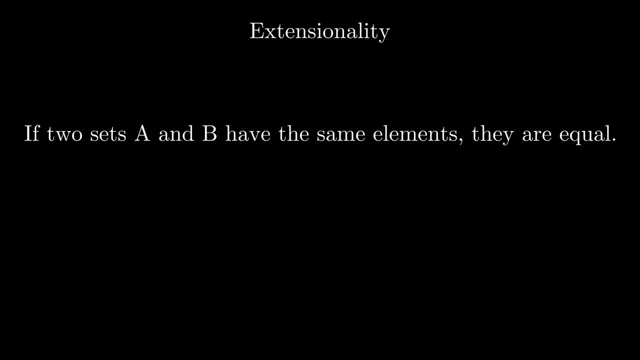 have the same elements, then they are equal, Or the axiom which declares the existence of an empty set. There exists a set, denoted by phi and called the empty set, which has no elements. But there is one axiom that has caused a lot of controversy: The axiom of choice. This is what it states. 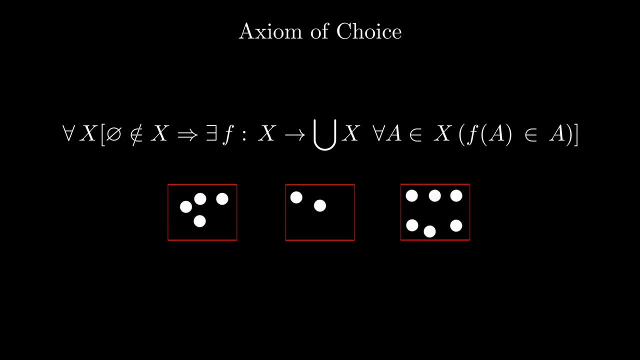 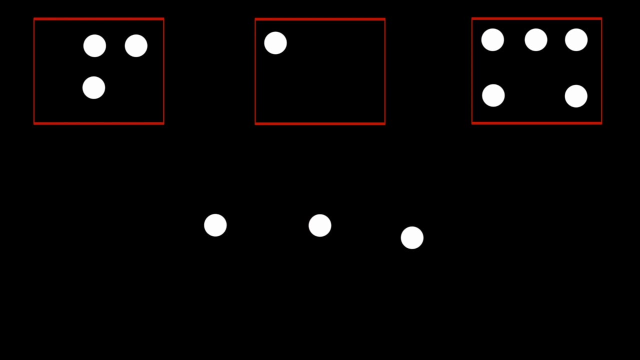 Alright. in human language it states that for any collection of non-empty sets, there is a way to choose exactly one element from each set, ie there is a choice function. It does not even sound like something we must assume. If you have the sets, simply take any. 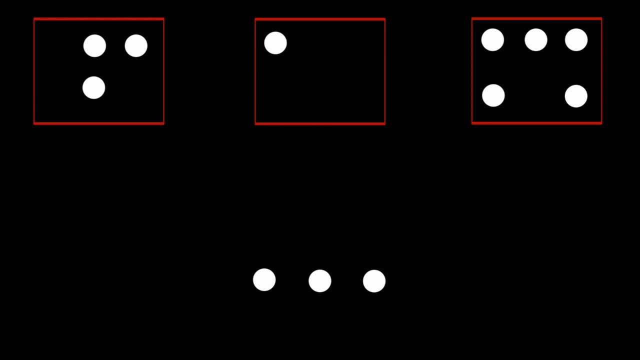 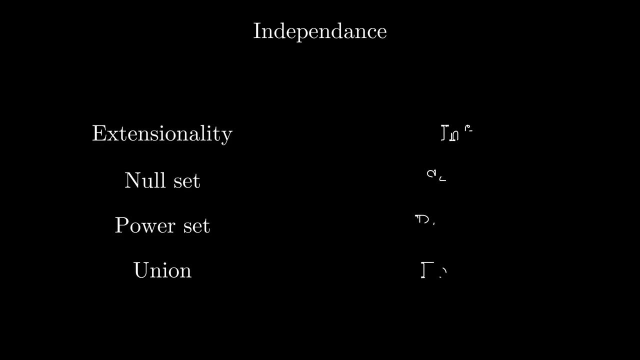 elements you want. So why even declare it as an axiom? Well, if you speak the strict language of first order logic, it turns out that the axiom of choice is independent of all other axioms. It means that if you use all the axioms from Zermelo-Fraenkel, 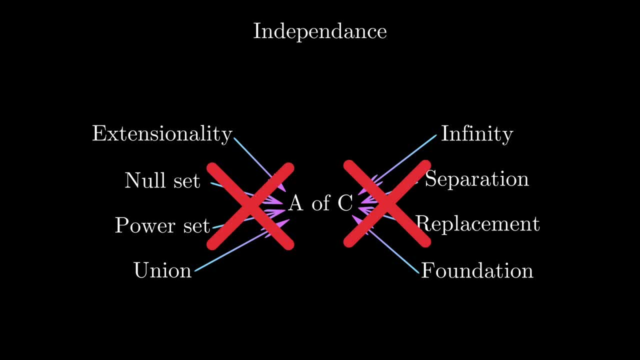 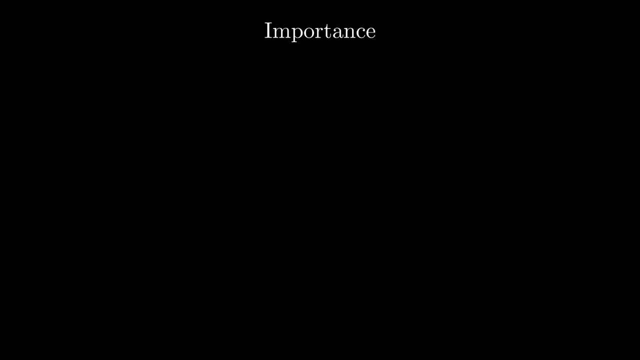 you can neither prove the axiom of choice is true nor that it is false. So the existence of a choice function is the actual option is not guaranteed by the other axioms. Right, but why is this axiom even important? Well, consider this statement: Every vector space has a basis. This 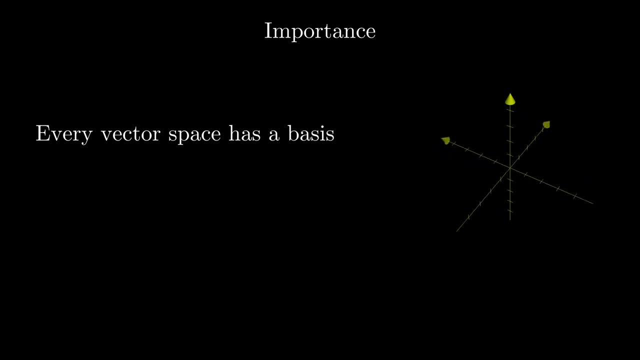 sounds remarkably obvious, something you should be able to prove from first principles. Actually, this is one of the most famous equivalents of the Zorn's lemma, which is equivalent to the axiom of choice. So if you don't have the axiom,